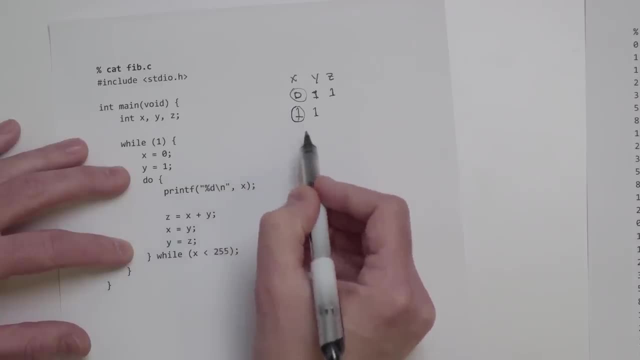 loop through again. We print out x, so x is 1.. And then we compute z again, So z is x plus y, So 1 plus 1 is 2.. And then we kind of shift things over, So x is equal to y. 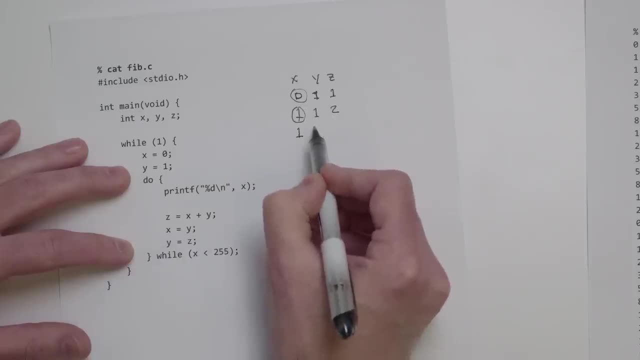 so x is equal to 1.. And then y is equal to z. z is 2, so now y becomes 2. And then we loop through again, because x is less than 255.. And here we print out: 1. We compute z. 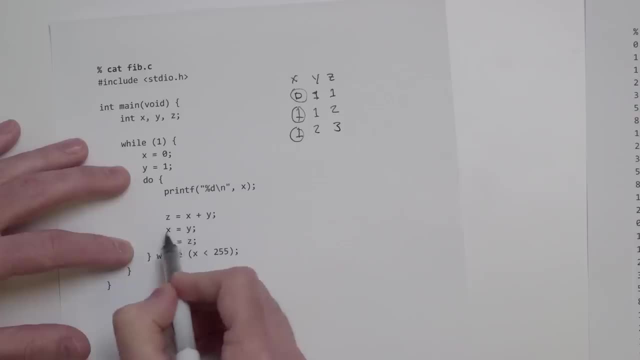 which is now 1 plus 2, is 3.. And then we kind of shift things over again, So the 2 shifts over here, the 3 shifts over here, So x equals y, y equals z, And then we loop through again. 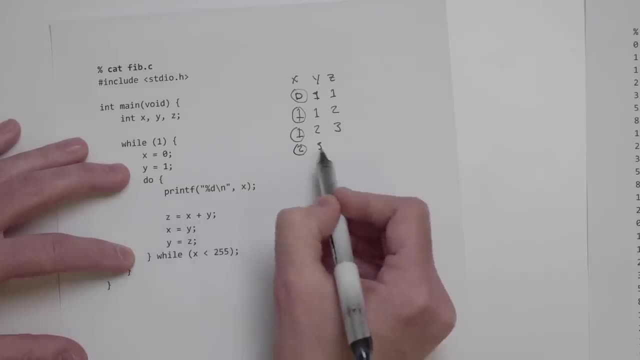 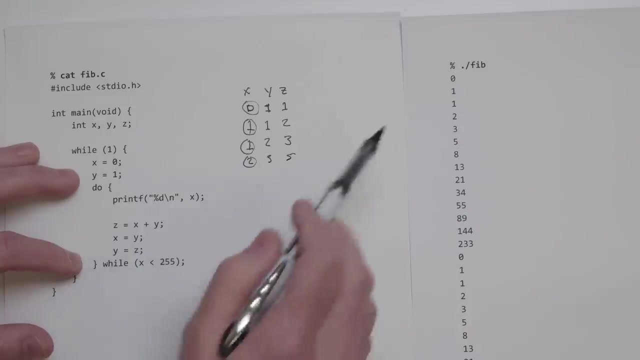 And here we print out the 2. We compute z as x plus y, so 2 plus 3 is 5.. And so on and so forth. And you can see, as we do this, we're printing out 0,, 1,, 1, 2, and so forth. So 0, 1, 1,. 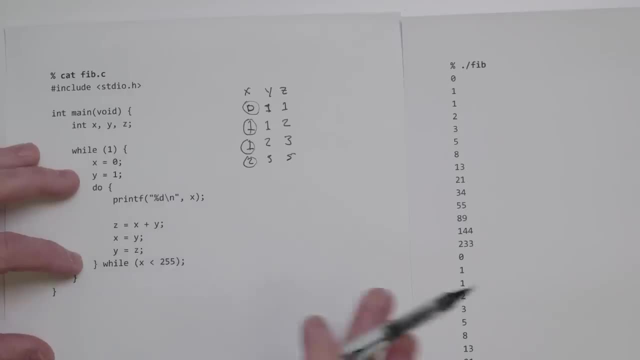 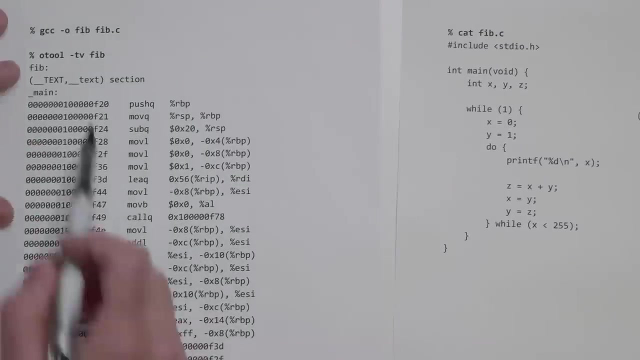 2. And it keeps going like that. So that's how this program works. prints out Fibonacci numbers. So what happens when we compile this? So if we compile it by running- this is the GNU C compiler, And I'm saying- the output file is just going to be a file called fib And 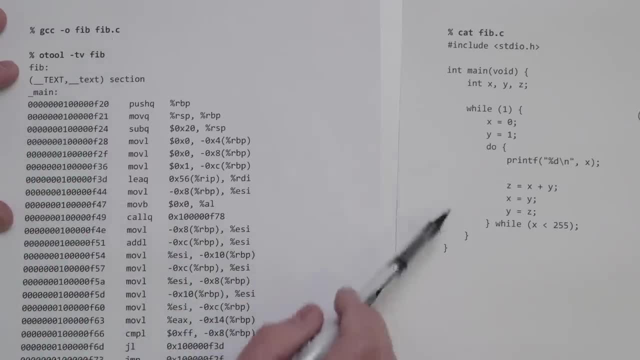 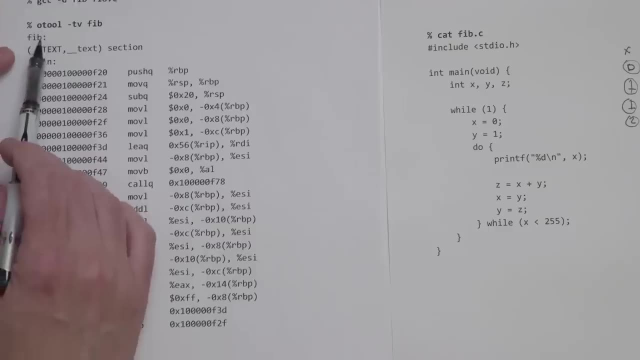 that'll be the executable that we'll run, And then the input is fibc, which is this code here that we just looked at. So if we compile it, then we can run it, But what I did here is actually disassemble it. So what this command does, this is just on my MacBook. 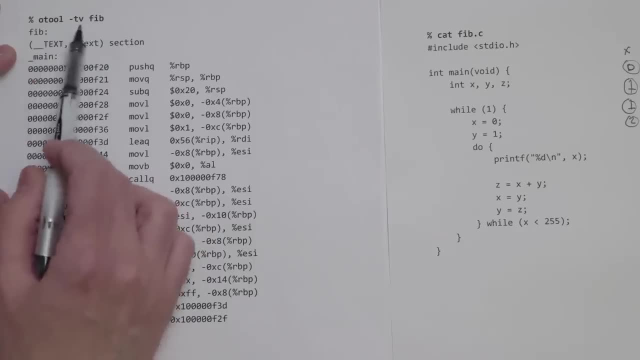 I don't know if this will work on other computers or whatever, but it worked. It worked on my MacBook And it prints out the machine language instructions that were compiled, And so we're looking at the compiled version of this program that we would run. 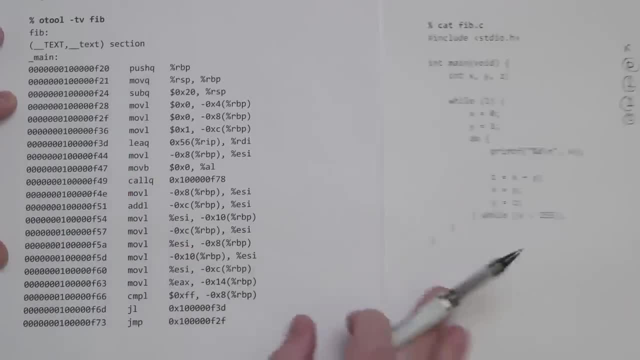 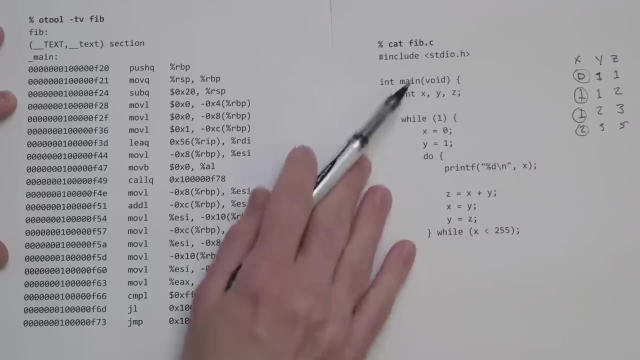 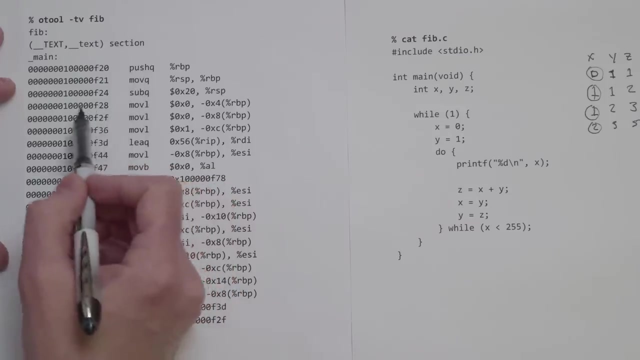 And so I want to walk through these instructions just to see if we can figure out which of these instructions correlate to what's going on in the original C program here. And so if we start here, the first couple of things here are just setting things up. These aren't. 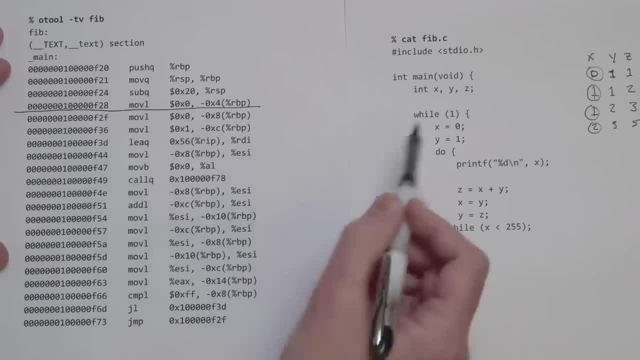 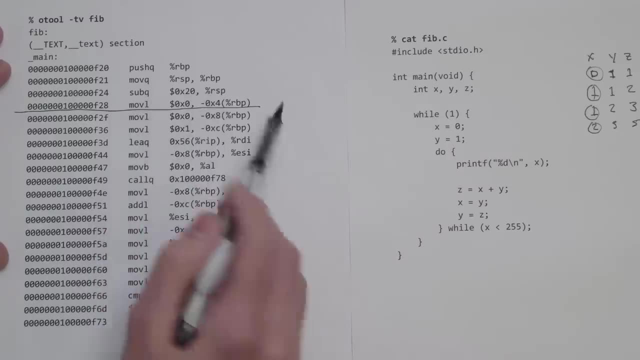 actually part. Everything up here isn't really part of what I wrote here. It's just kind of setting up the stack frame And this, I think, is a return value or something like that, which we aren't really doing anything with. So we'll just kind of ignore those for. 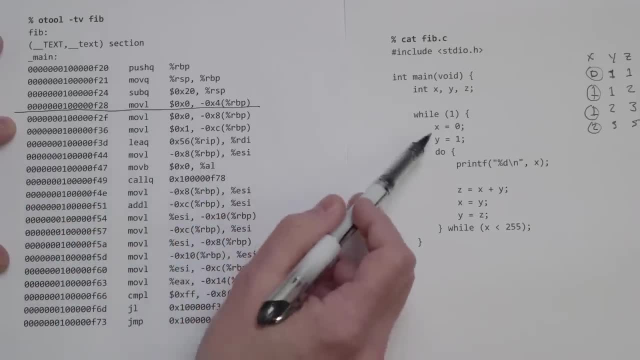 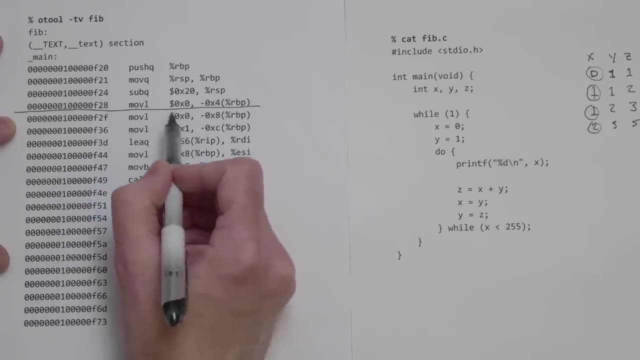 now. But here, here's where we actually get into the code that we wrote over here. So this first line here, this move long, is moving this value zero into this thing, which is actually an address offset. So rbp is the stack base pointer And this minus 8 is actually just an offset. So this is. 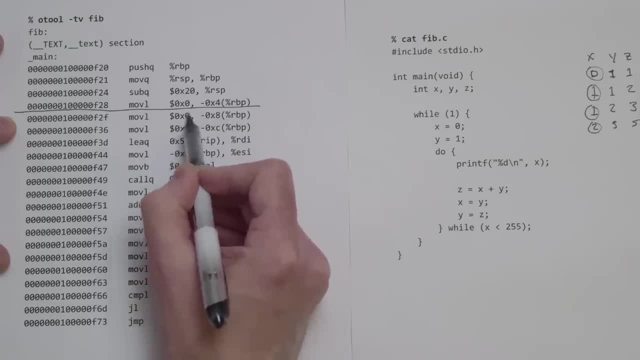 referring to a location in memory, And so we're putting a zero into this specific location in memory, which is exactly what we're doing here. We're saying x equals zero, And so what we can see is that x is actually this location in memory, this minus 0x8 offset from the stack base. 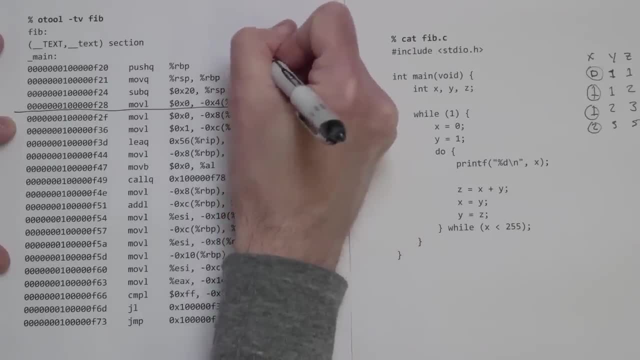 pointer. So over here I'll just write it Right. I'll write down that 0x8 is the variable x. So when we see it elsewhere in the program we'll know that that's x. So this line here is basically saying x equals 0.. So we're seeing. 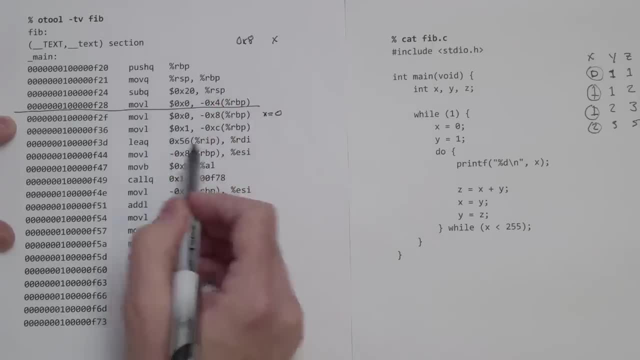 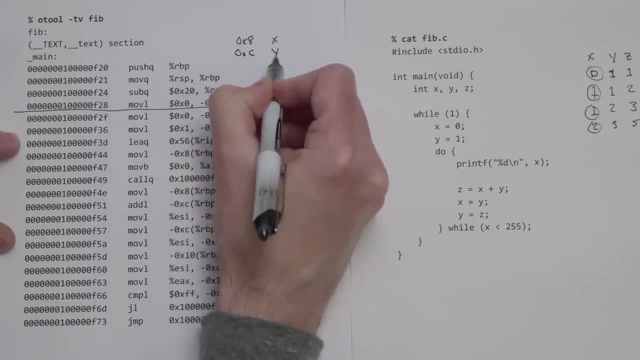 0 into 0x8, which is the memory location where x is The next line, is basically the same thing, except now we're putting 1 into this 0xc location. So here we're actually saying y equals 1. And 0xc refers to the variable y. 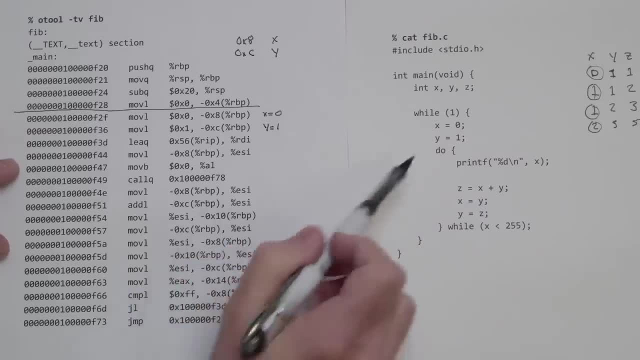 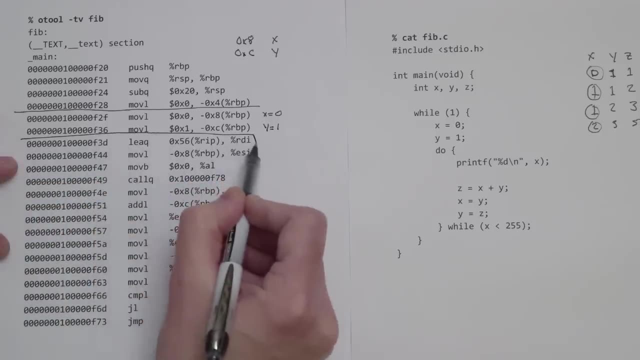 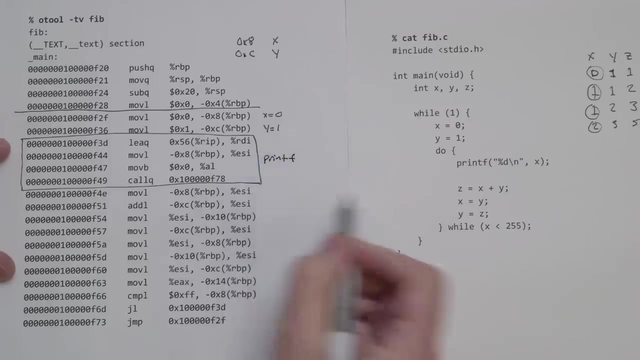 That's going to add up to 0x-y in the program over here. The next couple of lines. so now we enter this loop here. So the next couple of lines have to do with the printf, And so I'll just call out these four lines here that have to do with the printf. 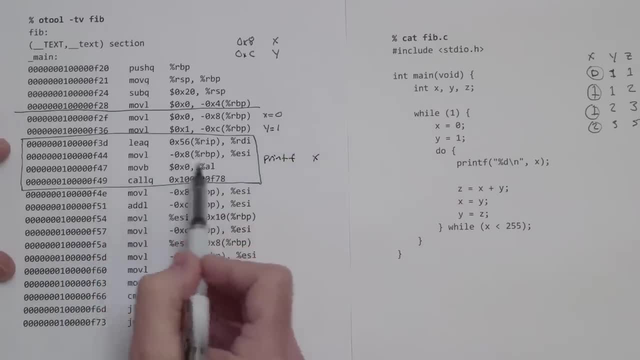 And we're printing the value of x And basically what these four lines are doing is it's setting up all the things and then calling this printf. I guess this is a memory address that's somewhere else in the program program that's not listed here. 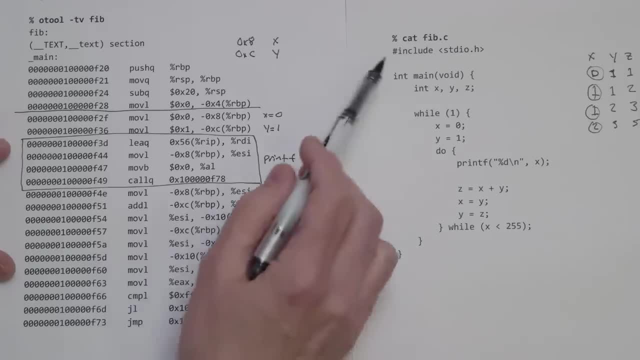 But this is presumably the printf function that's provided by the C standard library, And in order to call it we have to set some things up. I think this is probably the address of the string: the %d new line string And then, of course, 0x8,. we recognize that that's x, so we're printing x. 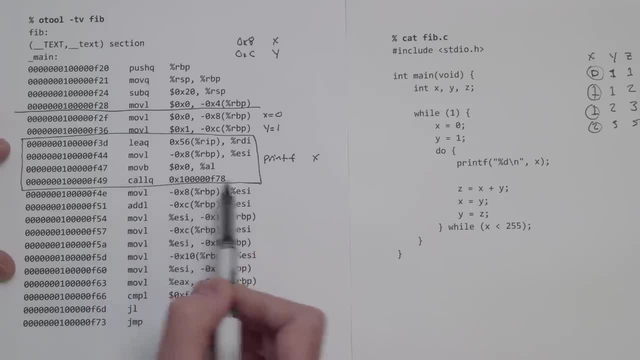 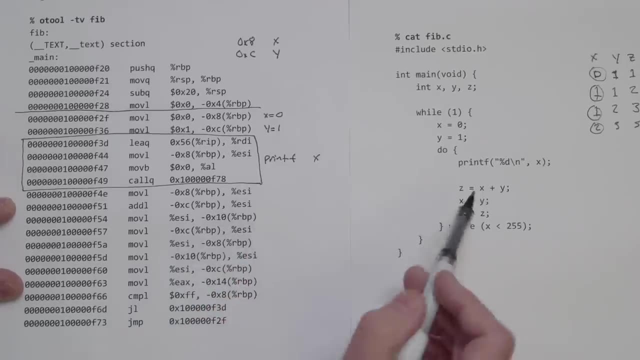 And then I'm not sure what this other thing is, and then the call actually makes the call to printf, So this sort of corresponds to that printf. So then after the printf we have this z equals x plus y, And that is actually these three lines. here are the z equals x plus y. 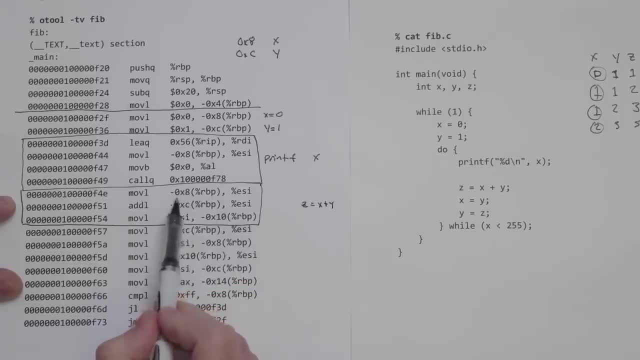 And the way this works is what we're doing is we're moving 8, 0x8, which is x, into this ESI register. So we're saying x goes into ESI, Okay. And then we're saying add, add the value of c. 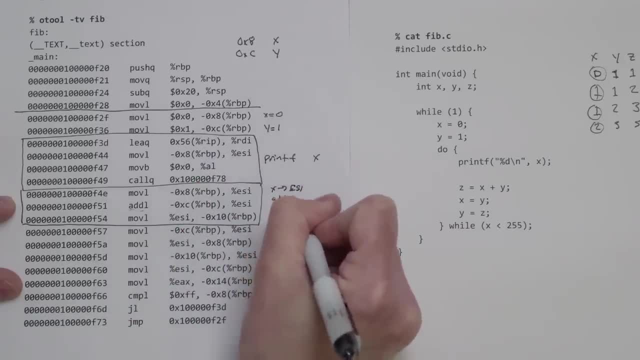 So we're saying: add y, add y to the value of ESI- And I probably can't read my handwriting here, getting a little messy, But basically what we're saying is: you know, x goes into the ESI register, and then we 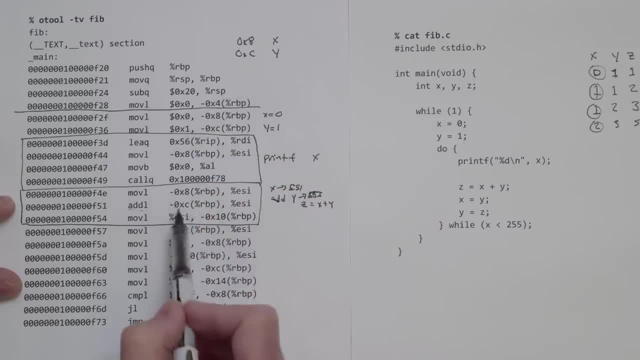 add the value of y- because 0xc is the memory location of y- to the ESI register And then take the value of ESI register and put it into this 0x10.. Okay, And 0x10 is a new memory location we haven't seen yet. 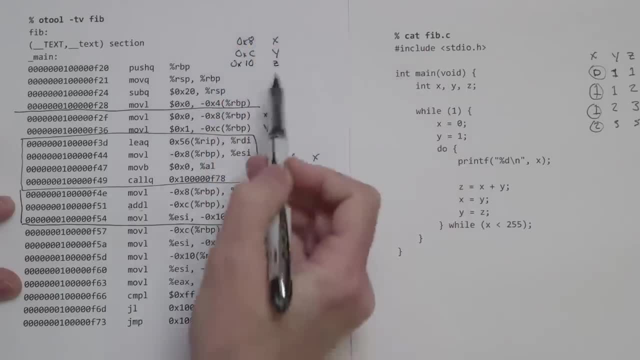 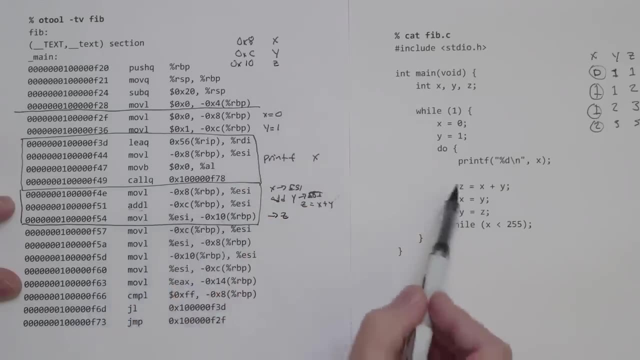 So 0x10, that's actually the memory location of z, And so then we just put this into z. So these three lines are basically doing the z equals x plus y. So we're getting x and putting it into ESI. 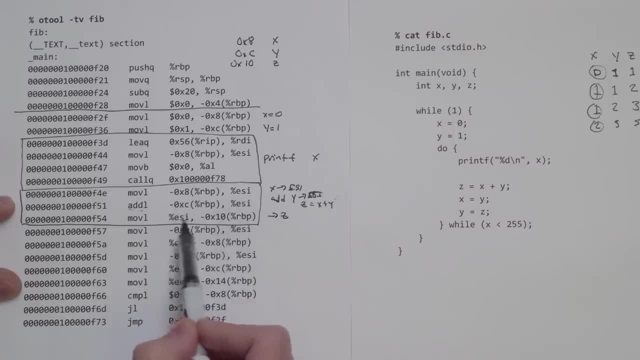 We're adding y to it And then we're putting the sum back into z. So then moving on The next two lines here, Okay, So we're taking the x equals y and again we're using this ESI register as kind of a. 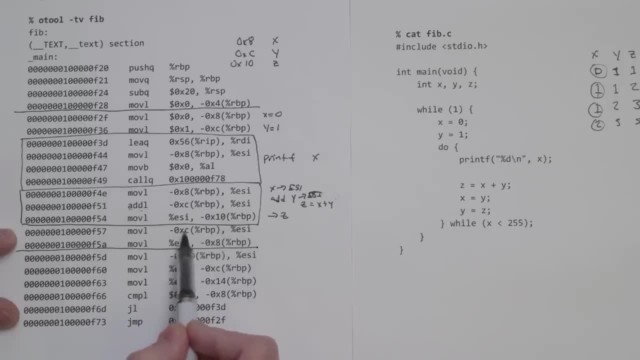 temporary location. And so we're taking 0xc, which is y, loading it into ESI, and then we're taking what's in ESI and putting it into 0x8.. So we're taking c and, yeah, we're taking y, putting it in ESI, and then we're taking 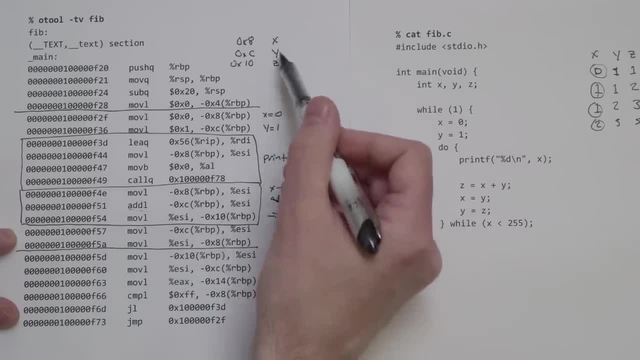 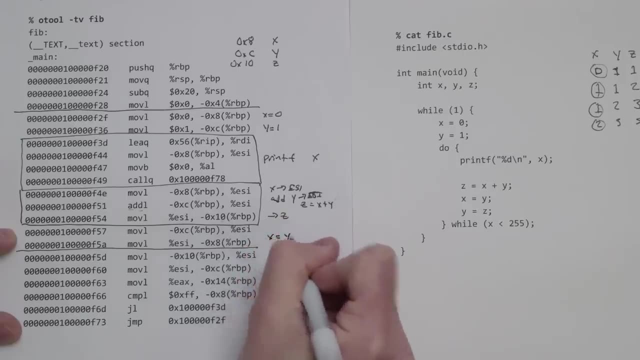 ESI and putting it in x. So from y to x, Or in other words, x equals y. We're setting x equal to y, And so this is the x equals y, And then the next two lines are basically the same thing, except now we're going from: 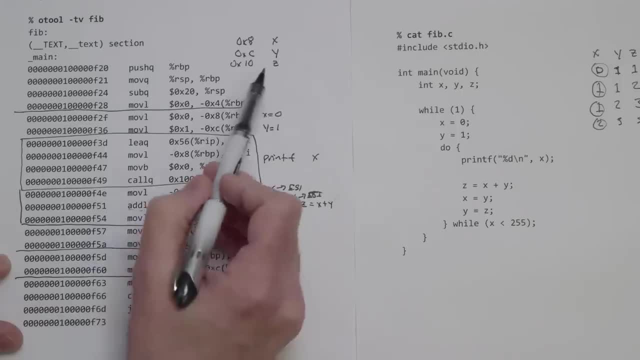 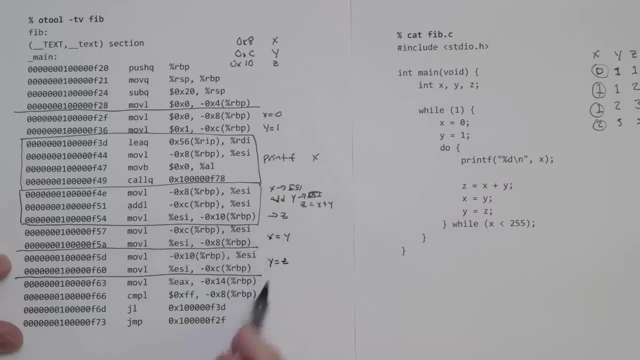 0x10 into 0xc, So we're going from z into y, or the way we write it here is: y equals z, So y equals z, This next line. I'm actually not sure what this line does, And so, if yeah, because this is the EAX register being moved into this other memory location. 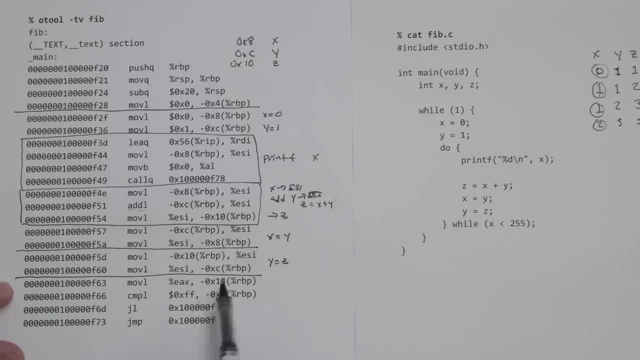 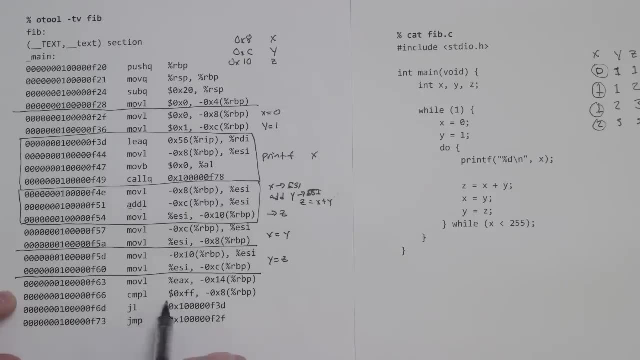 that we are not Using for anything else and we don't have any other variables to find here. I'm honestly not sure what this line is doing. So if you guys know, point it out in the comments. But after this line we do this comparison. 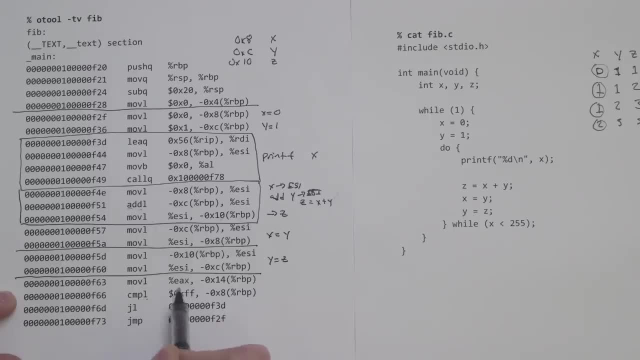 So this is the compare long value, And so we're comparing 0xff, which is the hexadecimal representation of 255.. We're comparing that to what's in the memory location, 0x8,, which is x. So we're comparing 255 and x. 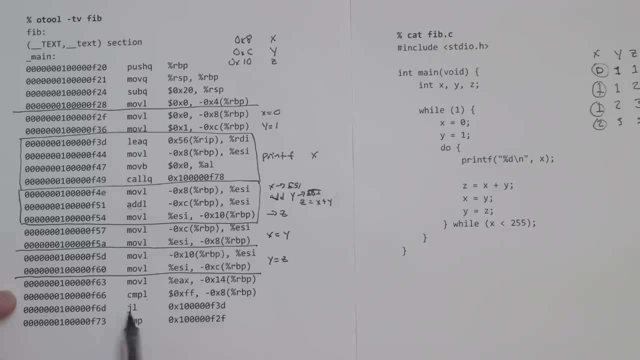 And we're saying jump x If less than. So jl is the jump if less than. based on this comparison, And the jump if less than is taking us to this address: f3d And f3d is up here, the first statement here. that was part of our printf. 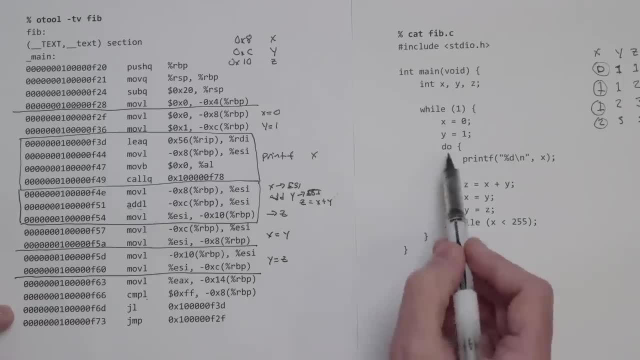 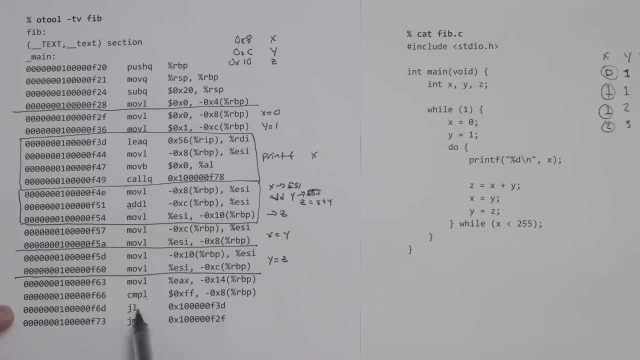 So if x is less than 255, we are going back up to the printf, which is what we're saying here. While x is less than 255, we stay in this loop. If it's not less than 255, then the flow. 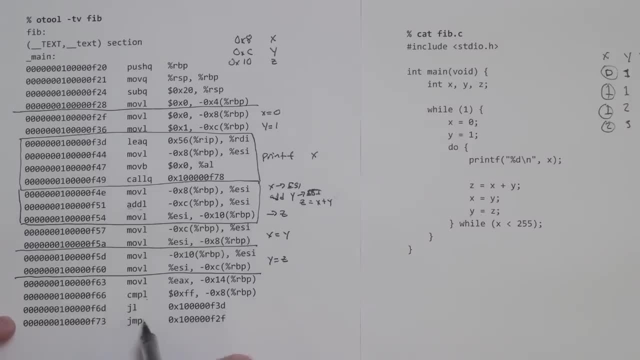 The program flow just jumps, Comes down to the next line here, which is just a jump, and this is an unconditional jump. We would always jump to f2f, and f2f is back here where we start with. the x equals 0.. 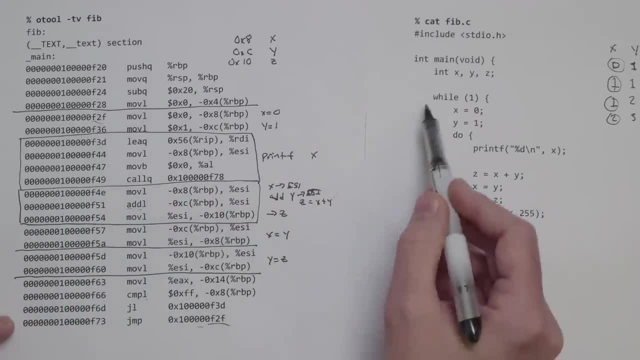 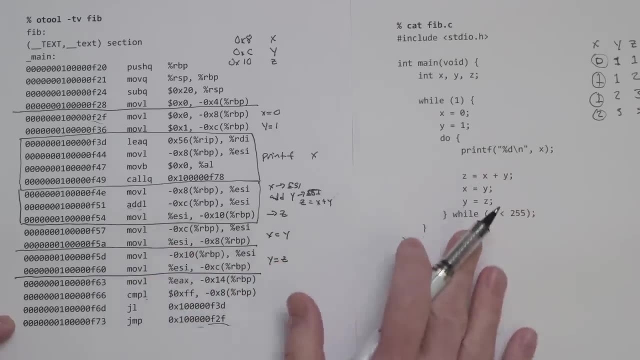 And, of course, once this loop is finished, we fall down here and we are back into this main loop that just goes on forever and ever. So you can see how, when we compile the C program, we end up with this machine code.